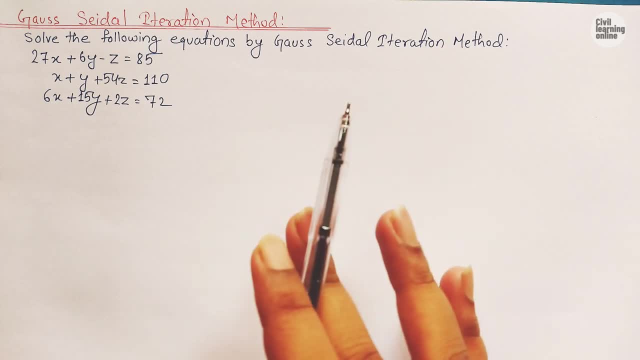 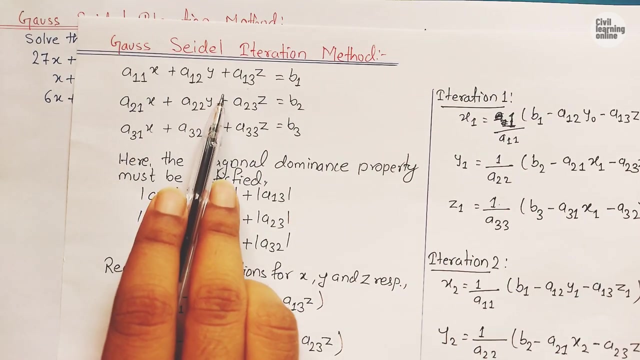 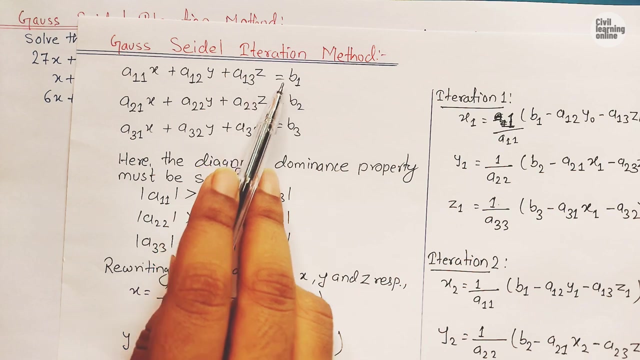 some arrangement here means we have to arrange this equation before solving this. it is because their equations must satisfy diagonal dominance property. and what is diagonal dominance property? let me show you so here we can see that. suppose we are provided with the equations in the form: a 1, 1 x, plus a 1, 2, y plus 8, 1, 3 z equals to b 1. similarly, a 2, 1 x. this is just. 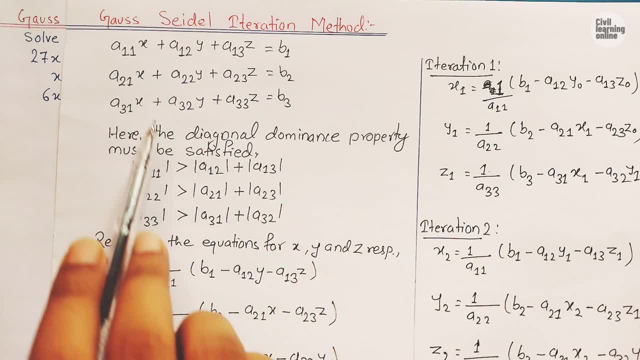 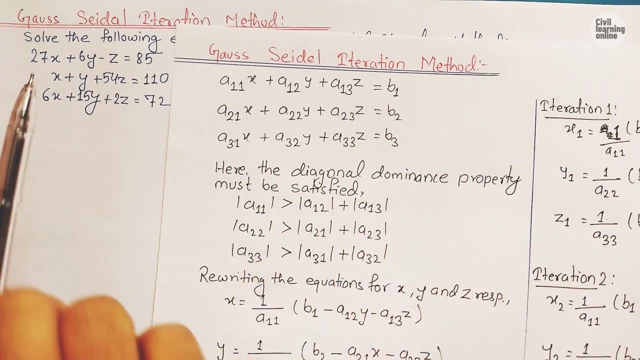 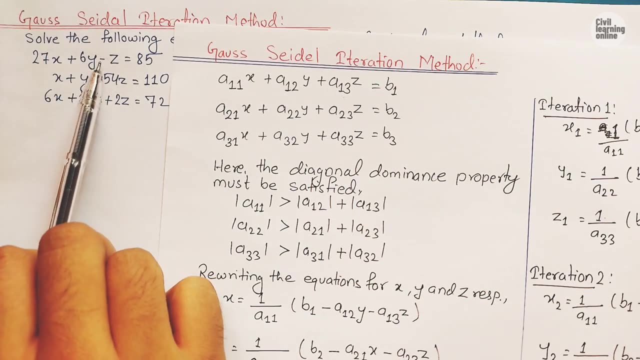 representing the coefficient or the magnitude of the variables. what happens here? in first row, a 1: 1 must be greater than the sum of other two coefficients. so here we can see that in first row, in first row, we have 27. 27 is greater than 6 plus 1. we do not, we will not consider minus sign, because 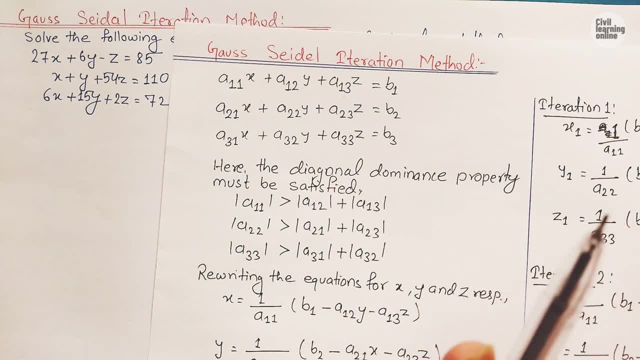 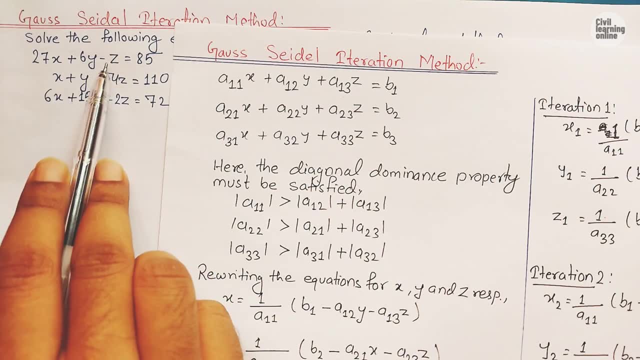 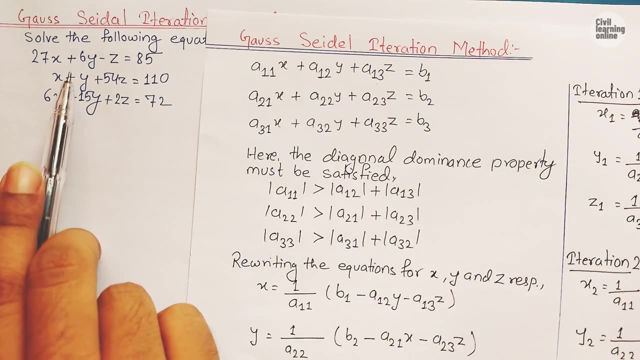 we will focus on the magnitude and or the coefficients which it carries. so we will ignore the signs and just do the addition of the coefficients. so 27 is greater than 6 and 6 plus 1, 7. okay, so first is set is first dominance property is satisfied. for second property, that is a 2, 2. 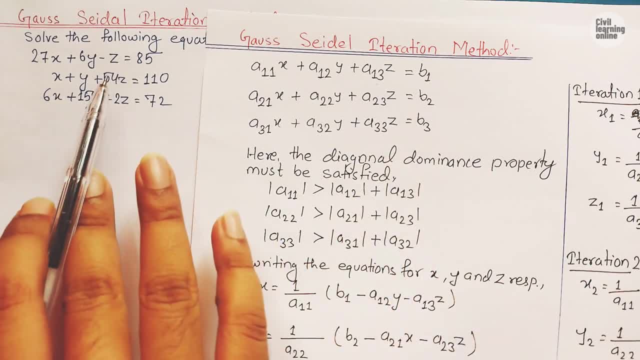 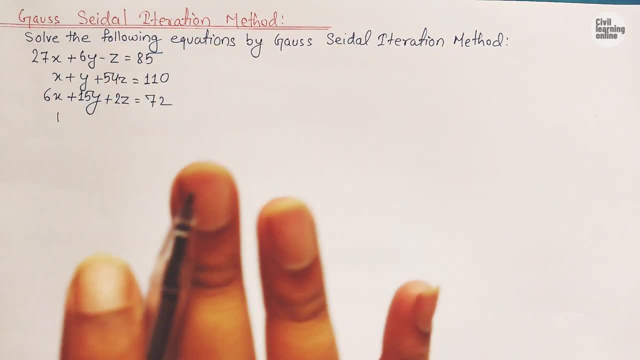 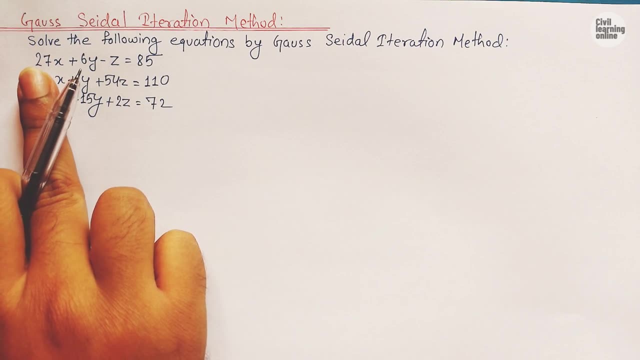 means the here. what we need to do is we have to do some arrangement. if we we need to rewrite these equations like this. see here: uh, i'm going to write here if it is already written in this form, suppose. uh, in the first equation, the coefficient of x, first x variable must be higher. 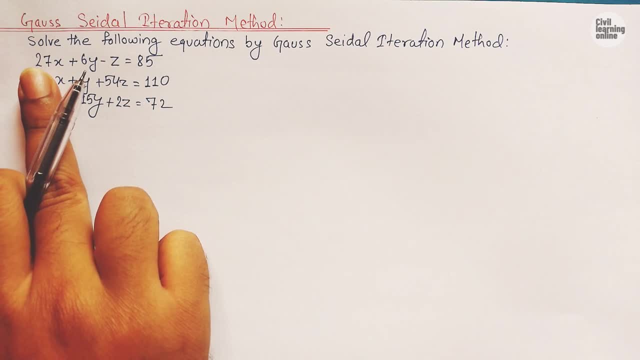 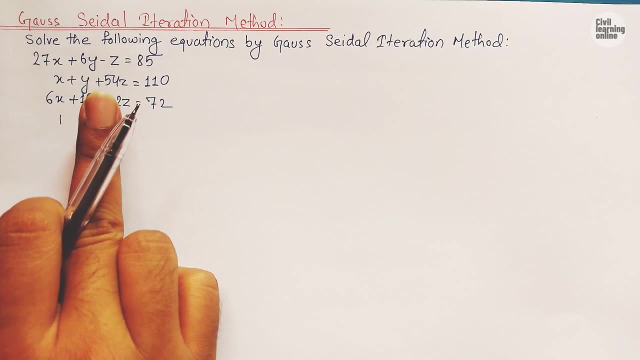 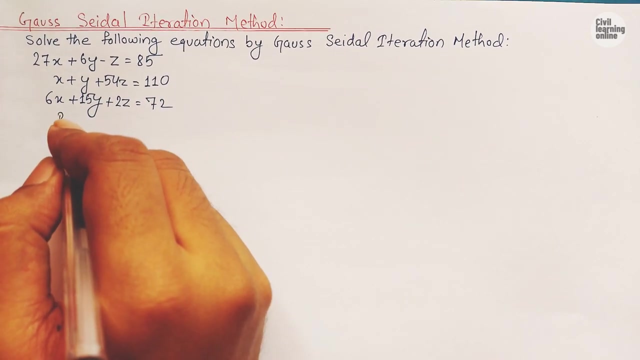 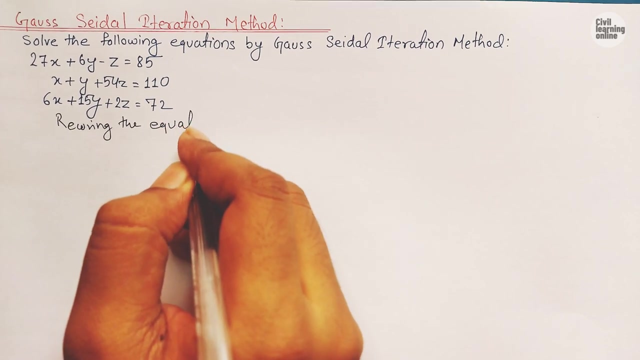 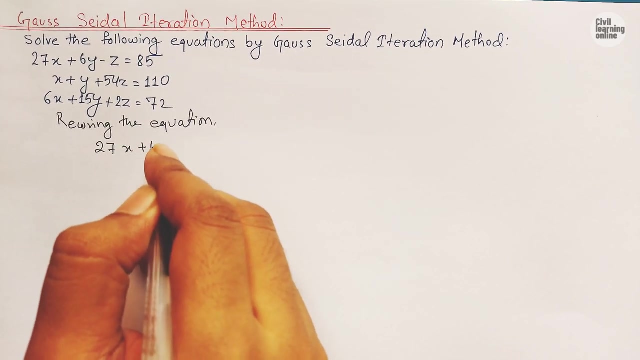 highest among other two variables. similarly, in the second equation, coefficient of y must be higher among other two variables. similarly, in third equation, the coefficients of z must be higher as compared to other two variables. so what we need to do here, we need some arrangement, so rewriting the equations. so so we one rewriting the equation, we will have 27 x plus 6, y minus z equals to 85. 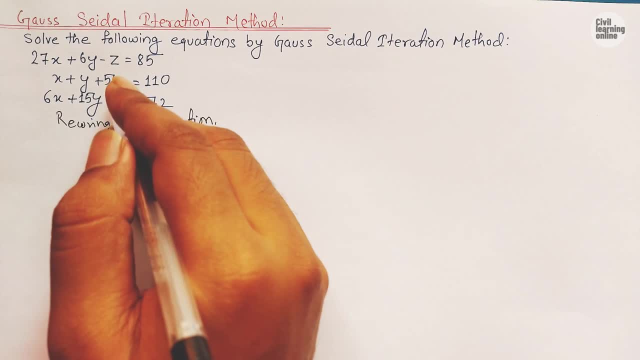 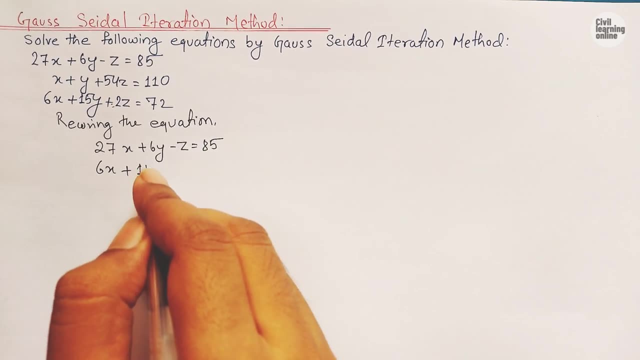 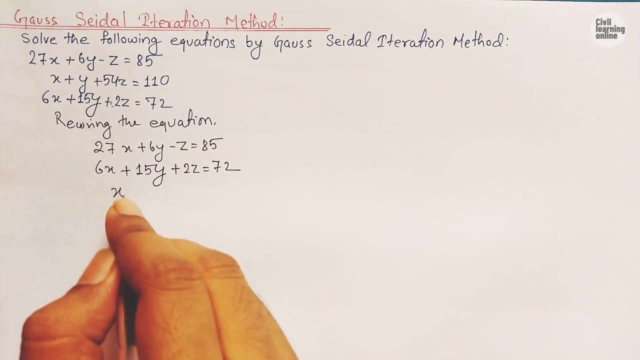 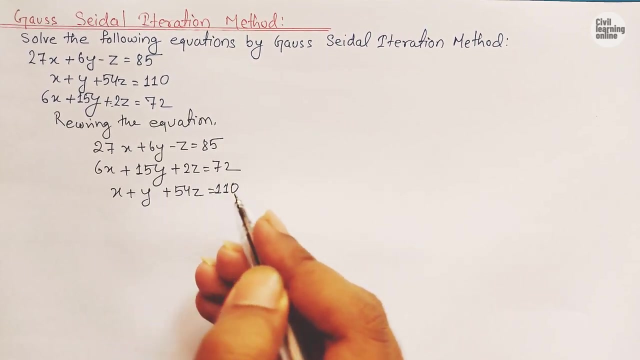 similarly, we need to rewrite this equation in the second position and this on third. see here what we will have here: 6 x plus fifteen y plus two z equals to to 72. similarly, we will have x plus y plus 54 z equals to 110. now we have just we have. 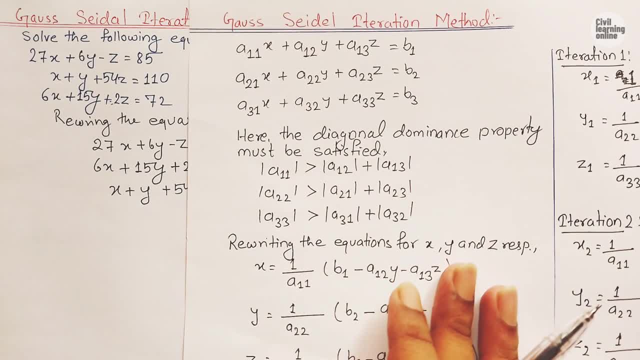 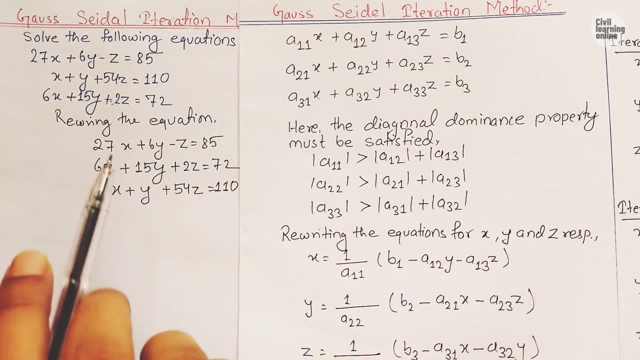 to check the diagonal dominance property in our mind. see, here we have a11, a22, a33. these three elements in each and every row are higher than the sum of the coefficient of two other variables. here 15 is greater than 6 plus 2- 8. similarly, 54 is greater than 1 plus 1- 2. here. 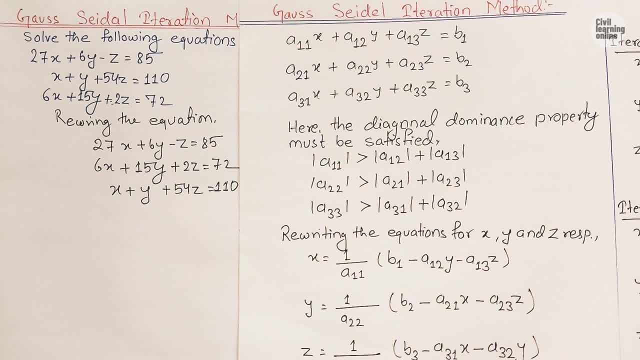 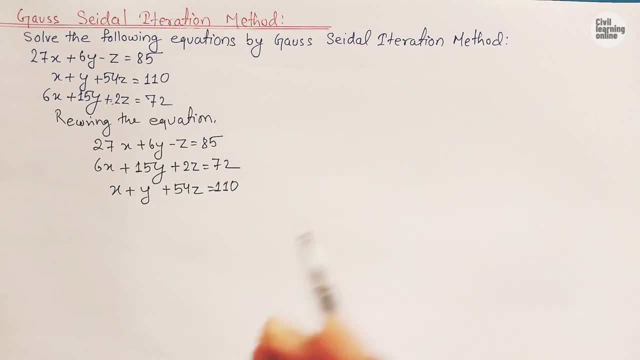 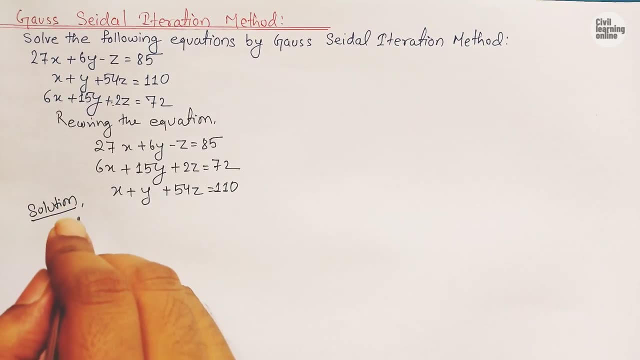 27 is greater than 6 plus 1, 7. okay, i hope you understood this. now what we need to do is we have to rewrite this equation again for the for x, y and z. so again, we will write here: solution: solution: writing: writing the the. 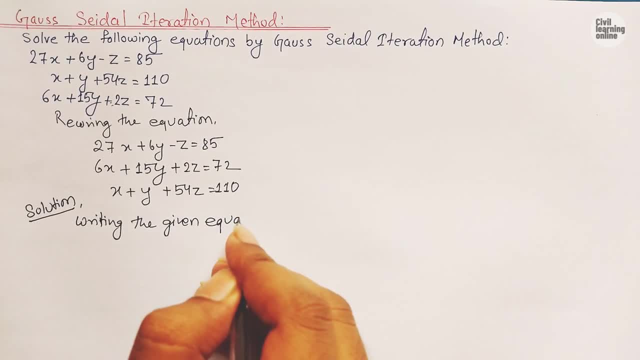 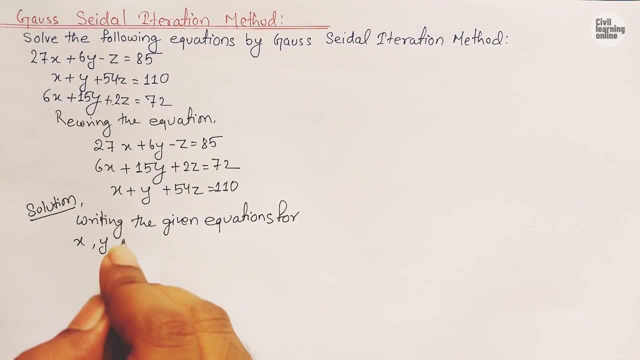 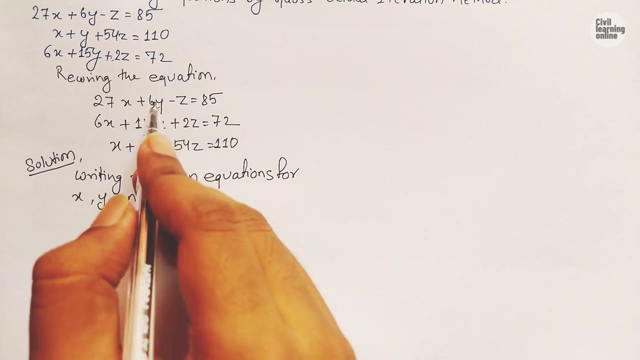 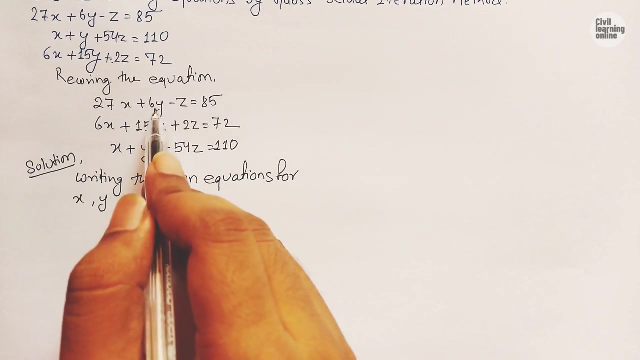 the given equations for x, y and z. so on writing the given equations for x, y and z. how we can write this, see here. what we need to do is we have to bring these two on other sides of equal equals to. so here it is 6 y, positive, so it will get minus. and here it is minus, so it will get positive, so we will have here. 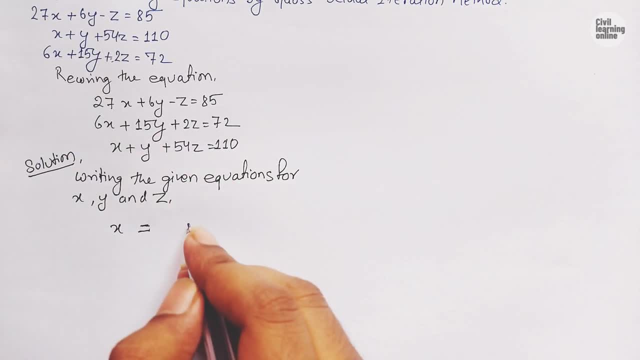 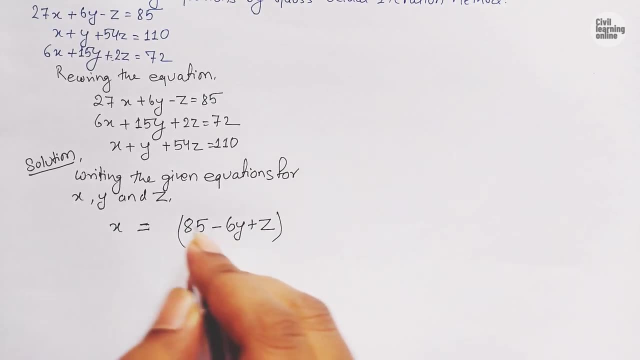 x equals to x equals to 85 minus 6, y plus z, and this whole divided by 27, this is for x. i hope you understood this. similarly, here we have to write for y, so for y. we will have here y equals to bring these two terms this side. so we will have 72 minus 2z minus 6x, so this is for x. 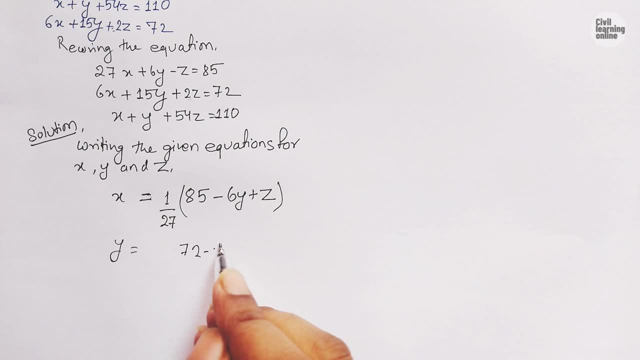 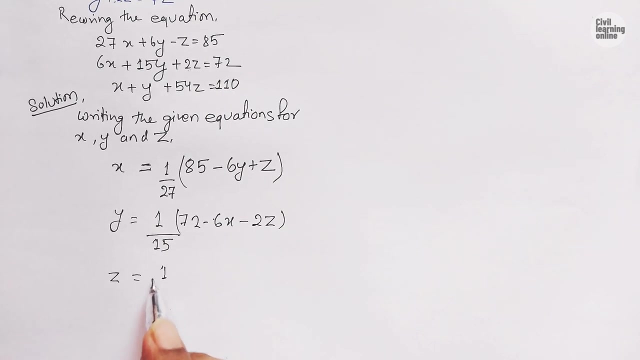 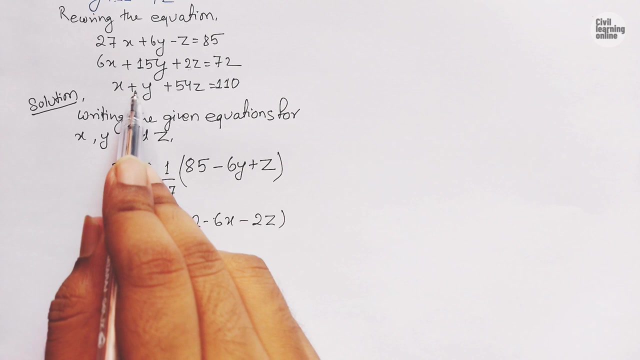 So I am going to write here 72 minus 6x minus 2z, and this divided by 15. this it is was for y. similarly, we will again write for z, so z equals to 1 by 54 times 1 by 54 times 110. 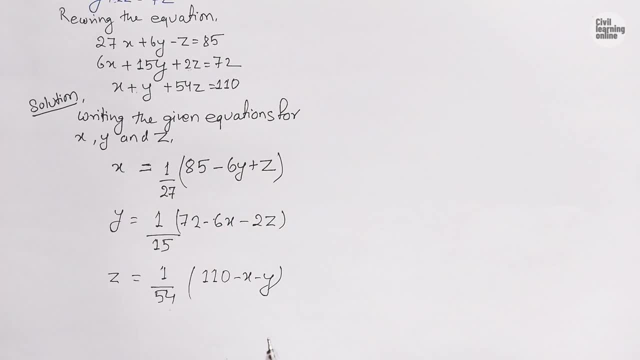 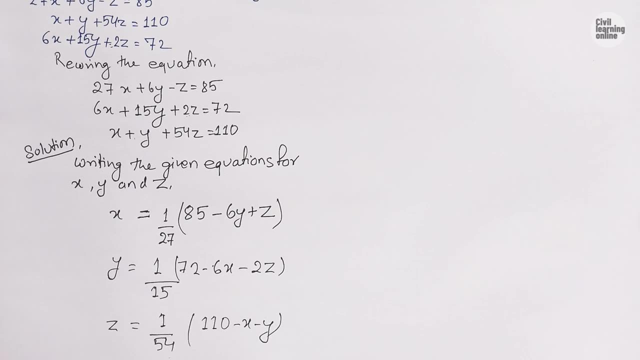 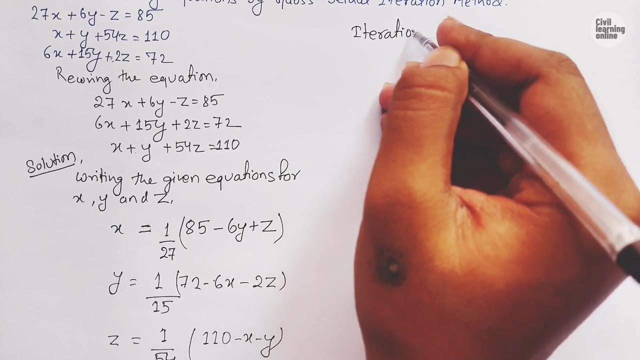 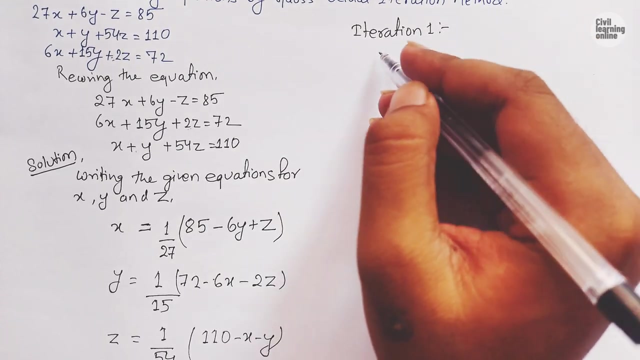 minus x minus y, minus x minus y. okay, these three equation we got for x, y and z. now we will proceed with the iterations. so how we are going to do iteration, see right here, iteration 1, iteration 1. for iteration 1, what we will do here, we will take, we will solve for x 1. 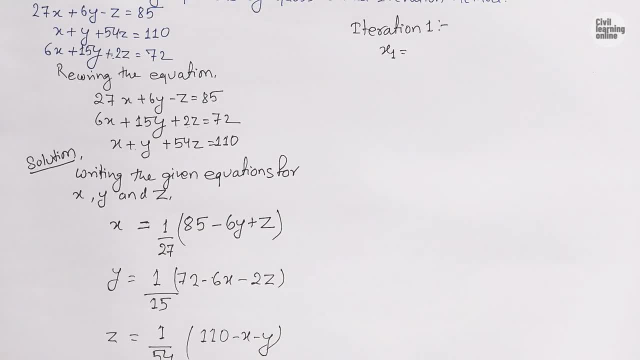 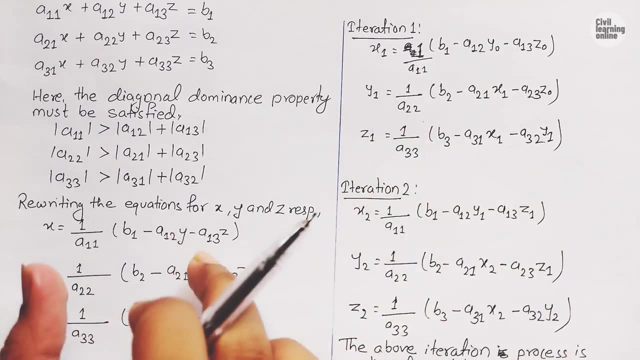 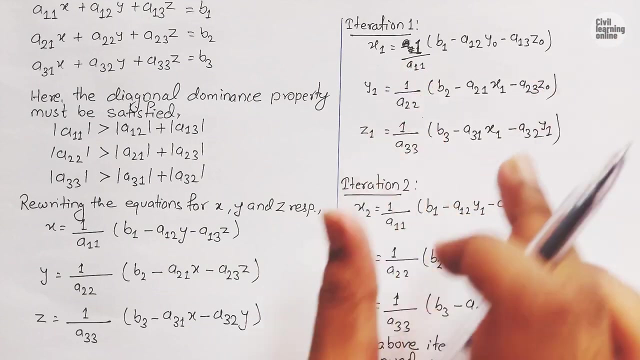 iteration 1 we will solve for x 1 and here if I tell, I will explain you the working rule- what happens here when we are calculating x 1? this is the same form which we which we got after solving for x, y and z. here I have written as it is. 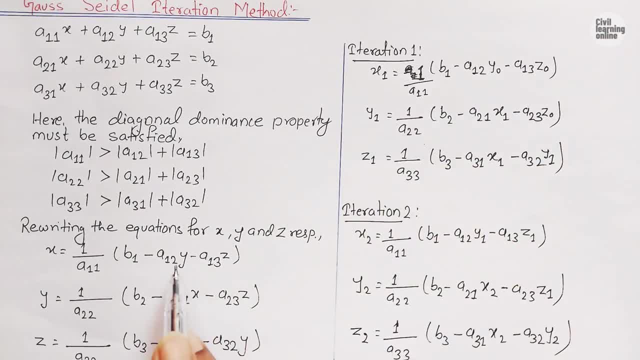 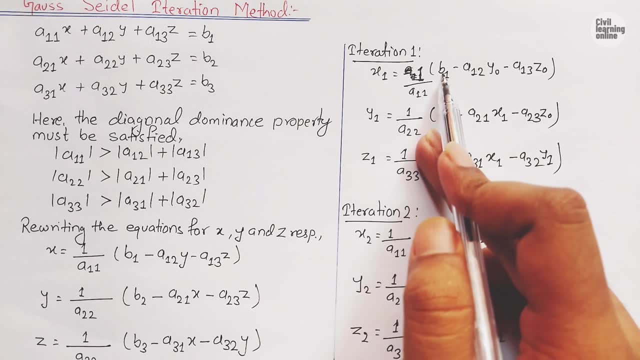 only the difference is what we will take. the value for y, z. okay, because we will be provided with the here: a, 8, a, 1, 2, a, 1, 3, a, b, 1 are the constants, but variables are y, naught, z naught. 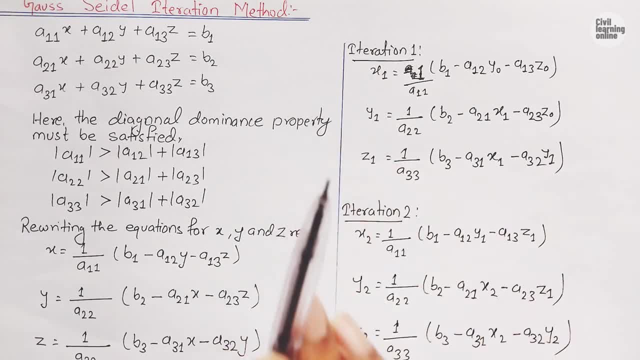 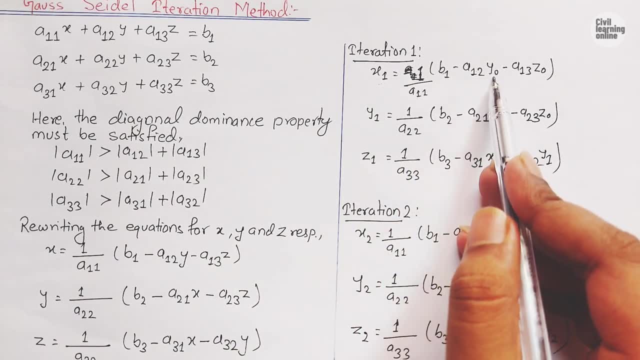 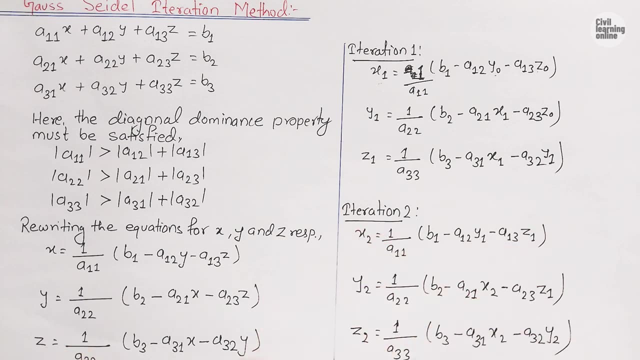 so what we will take, see here, I know, and only the problem is here we are letting these, we are telling it is the beginning or end of the problem. so I will take, whenever we are solving any problem based upon the g oui saddle iteration method, and we are when we are finding x one, we will take y note z. 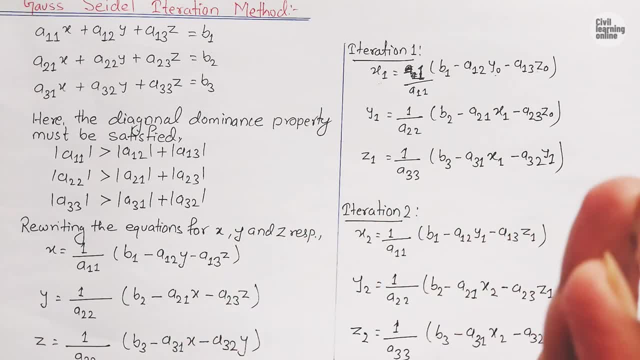 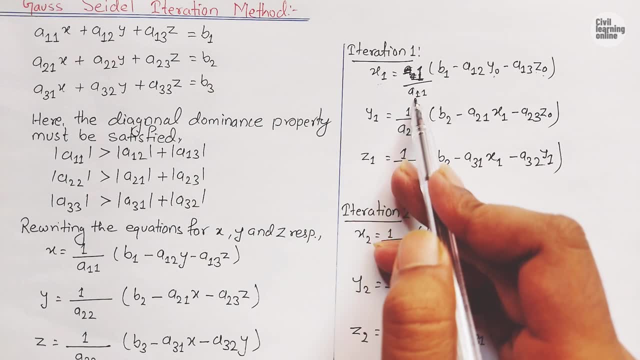 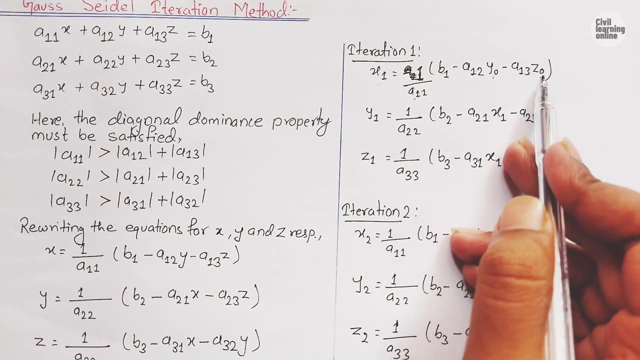 net equals to 0-1. remember we will take Y and Z equals to 0-1. the initial iteration elements are not given in the problem. we will proceed with taking 0 value. ok, so here we will take 0, 0.. but we will not have the value of this variable, so we will proceed with 0, and once we get the 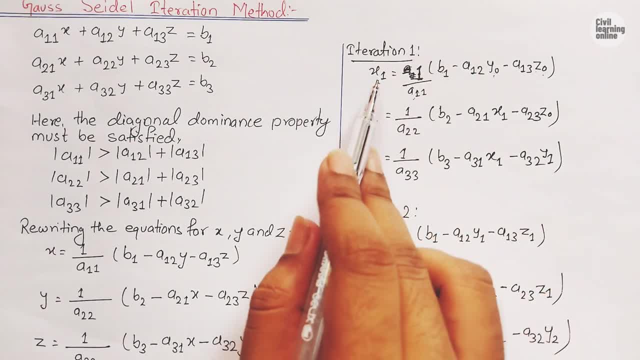 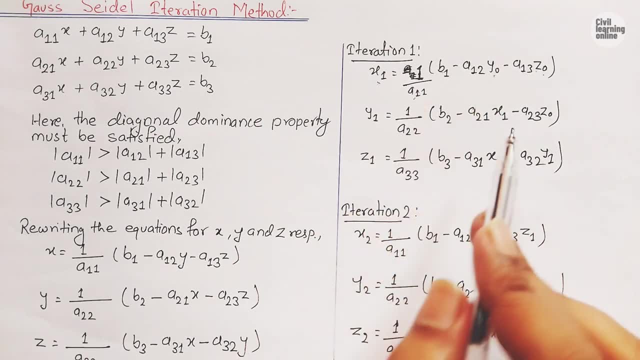 value of x1. what we will do, we will pro we will supply this x1 value to y1 because in in well, solving for y, we will see x in that equation also. so here we will provide the value we got. what we got means recent value is provided to the uh. succeeding equation succeeding. 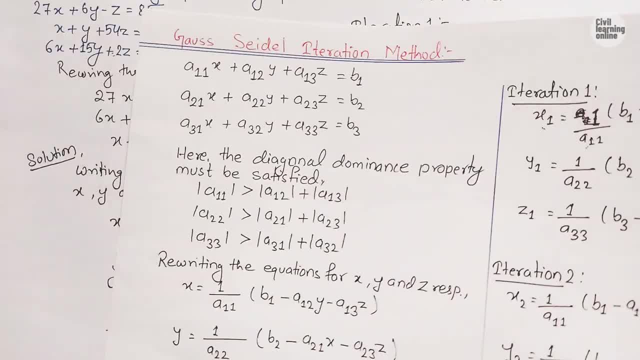 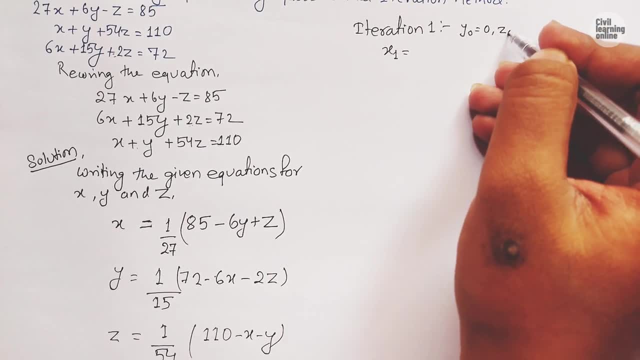 step. also, we can say that. so, uh, this is what we are going to do here. so we will take, for iteration 1, we will take y naught equals to 0 and z naught equals to 0, and we have x equals to 1 by 27. 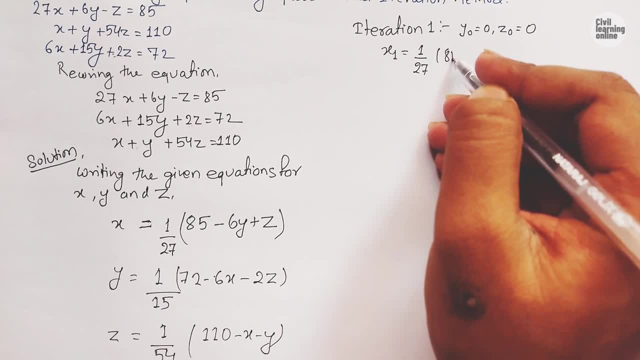 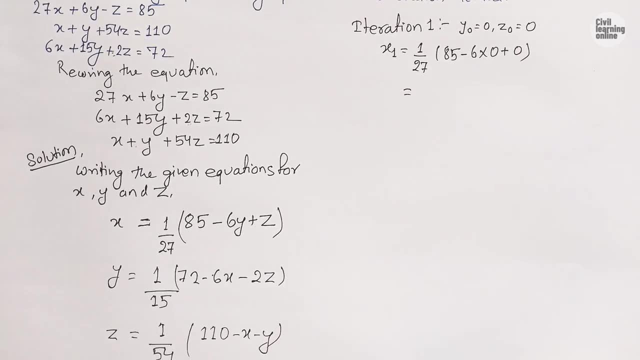 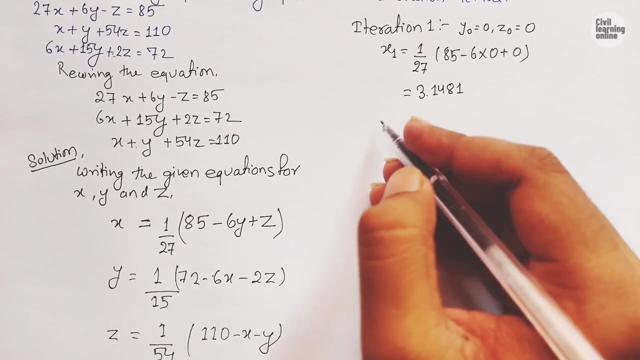 1 by 27 times 85 minus 6 times 0 plus z means 0. on solving this, we will get the value of x1 as 3.148. okay, similarly we will do for y1. for y1 we we have equation 1 by. 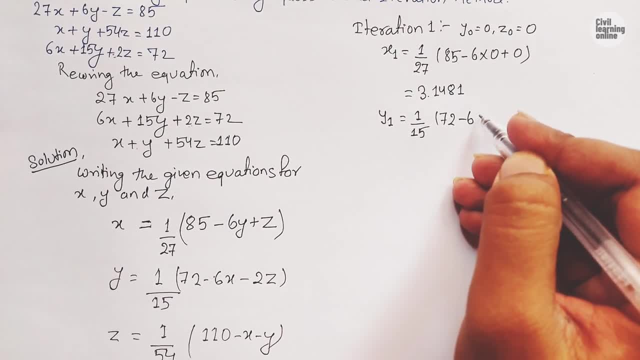 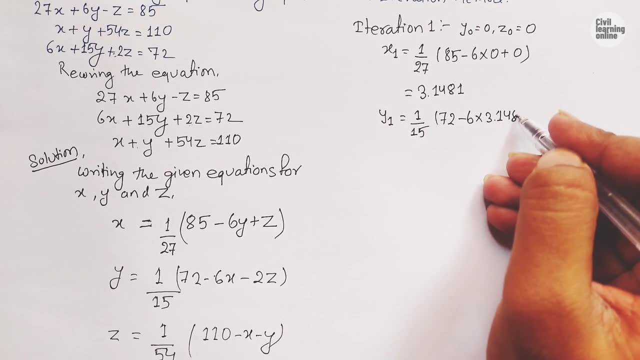 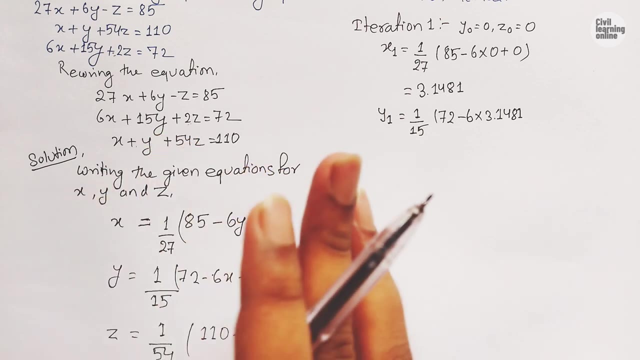 15 times 72 minus 6. and this time we will not take x naught, we will take the value which we recently got, that is, 3.1481. this is the difference between the gauss sedal iteration method and jacobi's iteration method, or gauss- jacobi's iteration method in gauss- jacobi's iteration. 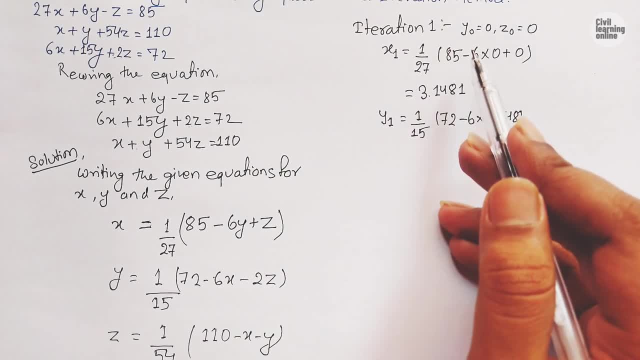 method what we had? the difference between the gauss jacobi's iteration method and the zacovis iteration method. what we had the done here? we would have taken x naught equals to 0, y naught equals to 0, z naught equals to 0, but 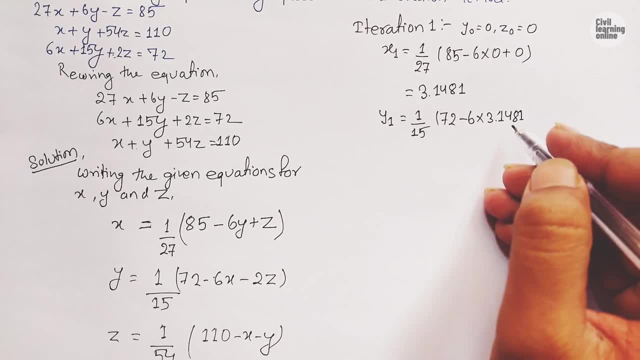 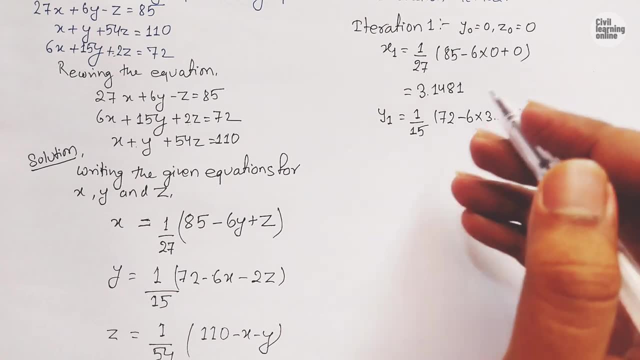 here we will take the recent value for x1, y1 and z1. so here, 6 times 3.1481. you can take up to 3 or 4 decimal places in this problem. i am taking up to 3 to 4 decimal places. so here we have taken. 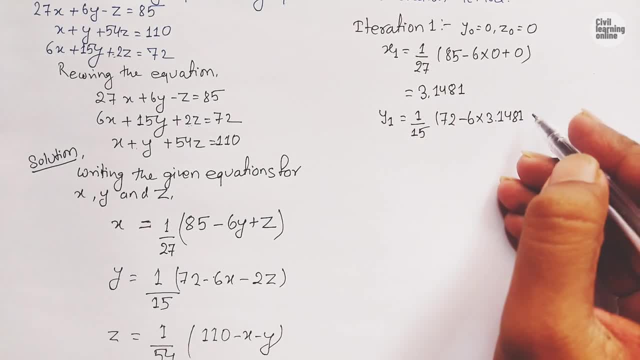 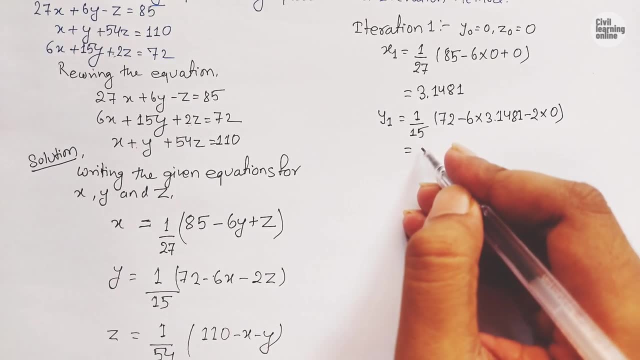 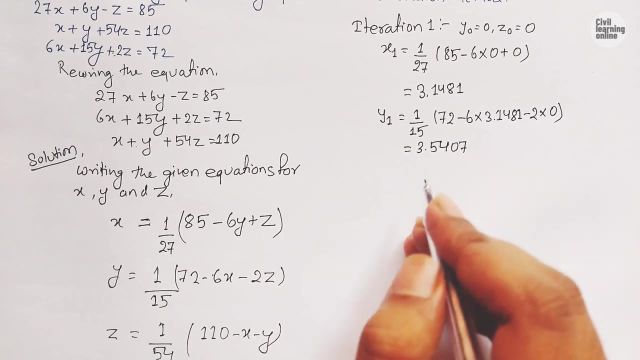 4 decimal places means after decimal. we will. i am taking 4 digits. so here, 2 times z, naught is 0. on solving this we will get the value of y1 equals to 3.5407. i am not doing the calculation. i have already calculated the value. but you can, once you, calculate this value using calculator. 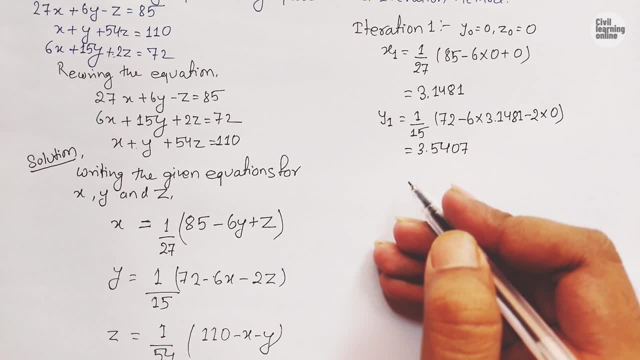 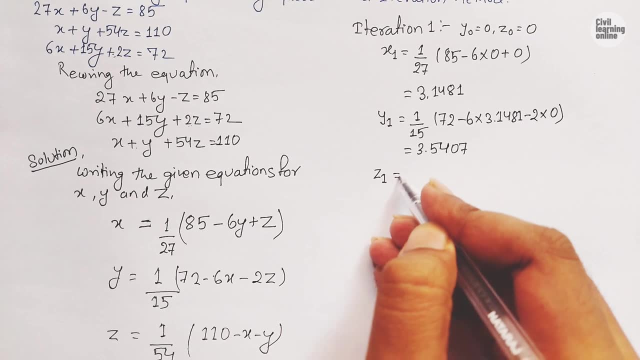 you will get the same values. in some position you i may have round off, but that won't create any kind of problem because at the end you will get the value. similar answer. okay, so z1 equals to 1 by 54. 1 by 54. 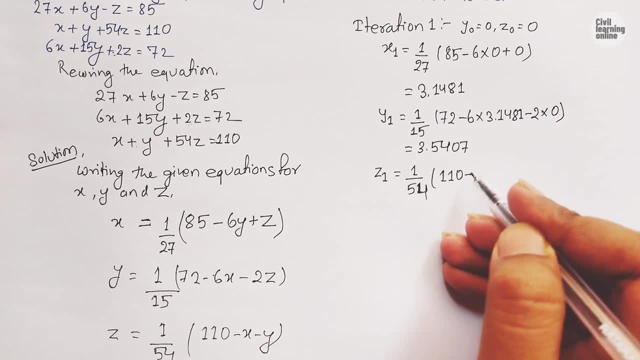 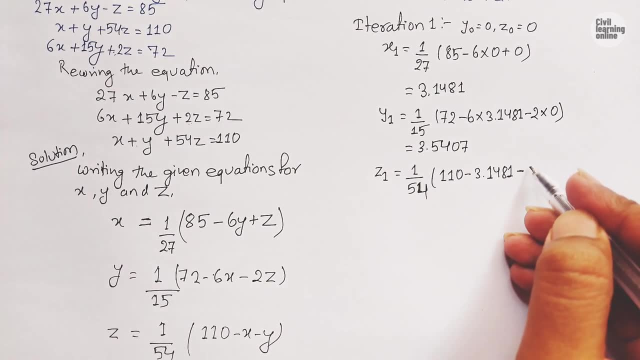 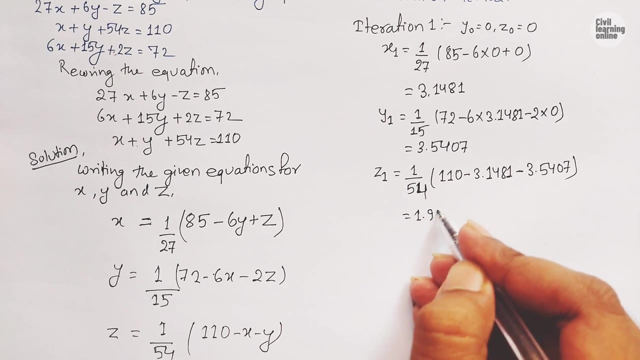 times 110 minus x is 3.1481. minus y is 3.5407. on solving this, we will get the value of z1 equals to 1.9131. this was our first iteration. now for second iteration. what we will do? we will. 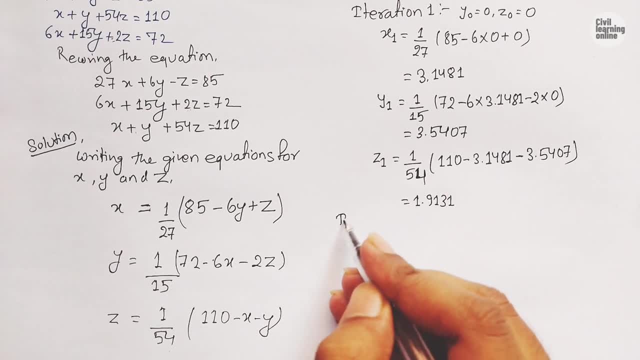 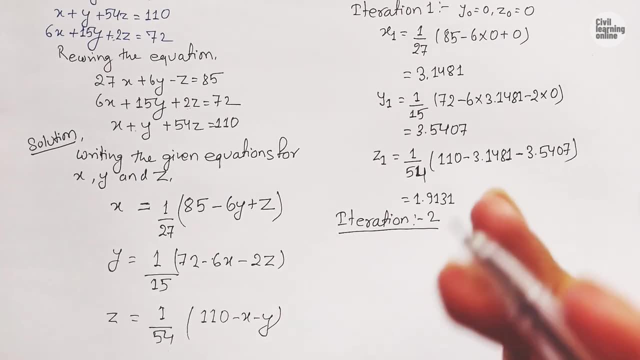 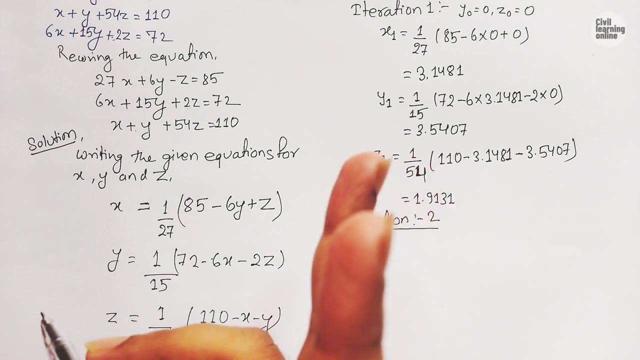 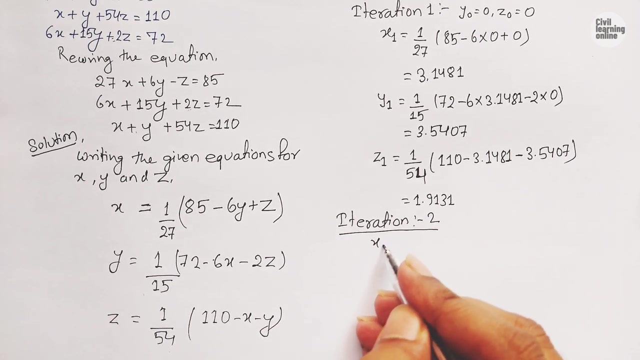 use these values for in second iteration. so see here iteration 2, and we have to keep doing the iteration until similar value. in two respective iteration we must give the same value of x, y and z. if we start getting that value then we will stop doing iteration. so for iteration 2 we have: x2 equals to one by 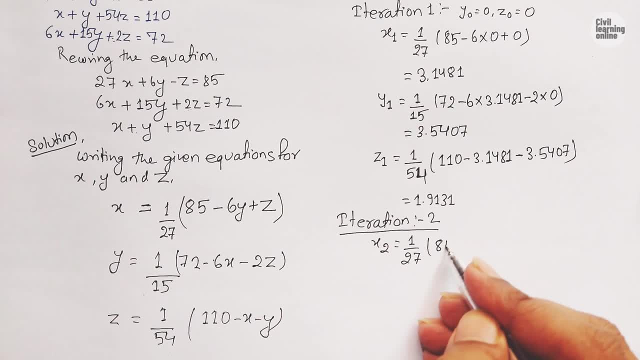 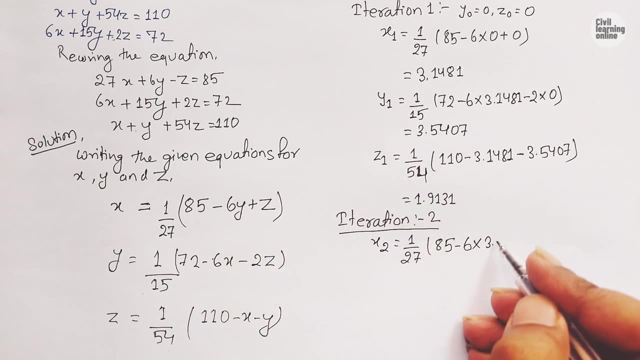 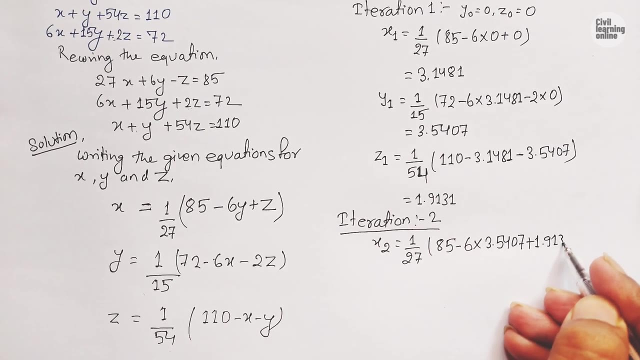 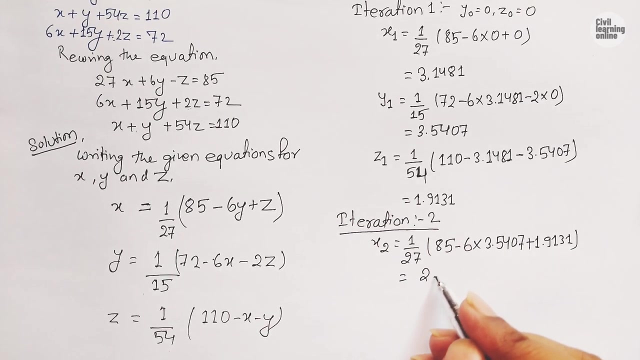 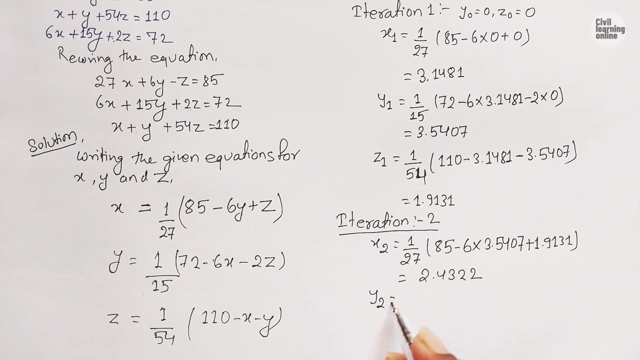 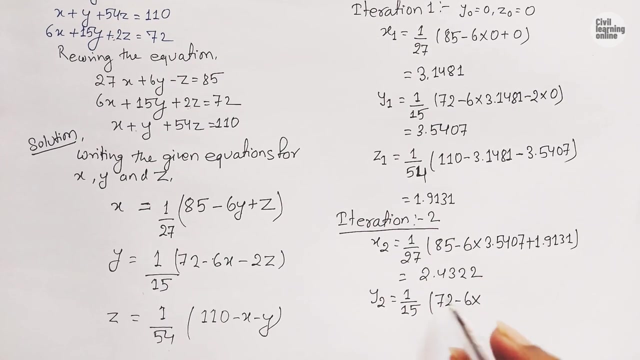 27 times 85-6 times y. value is 3 point in place of y. we will use this value. so 3.5407 plus z is 1.9131. okay, so on solving this, we will get x2 equals to ah 2.4322. similarly, for y2, y2 we will have 1 upon 15 times 72 minus 6 times x1. ah means 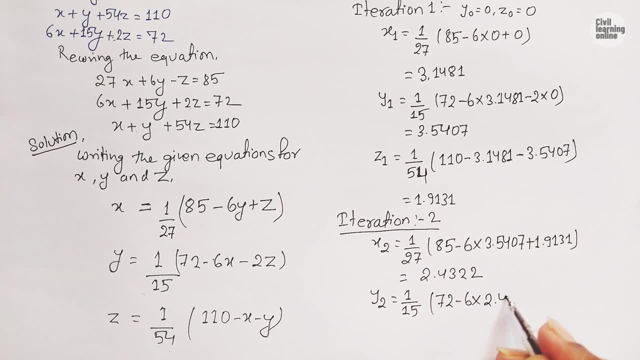 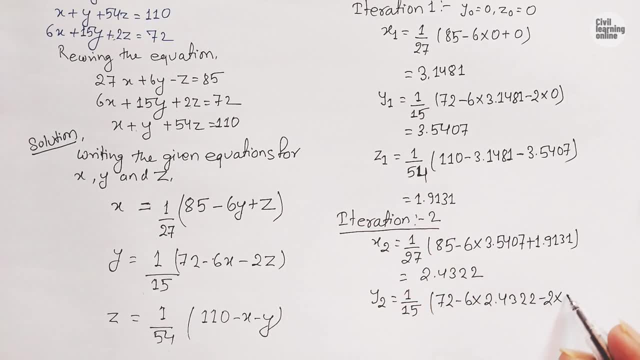 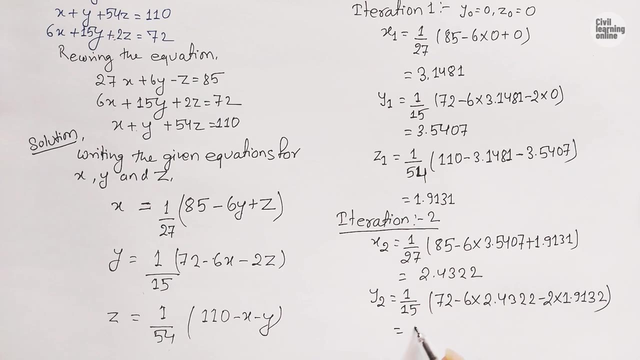 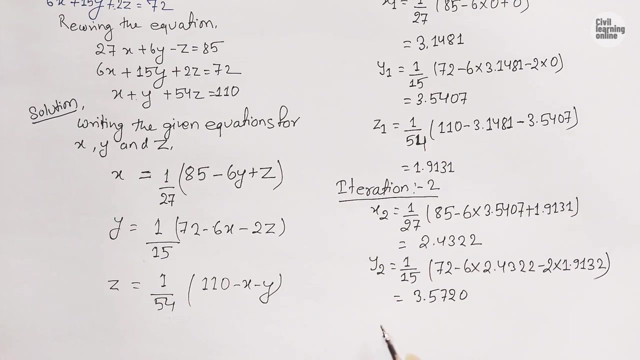 we will. this time we will use the recent value of x, that is, 2.4322 minus 2 times, and z value, z value. we will use this value: 9132. okay, on solving this, we will get the value of y2 equals to 3.5720. again for z2. for z2, what? 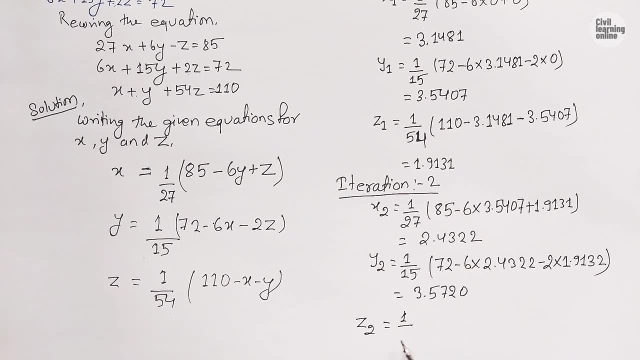 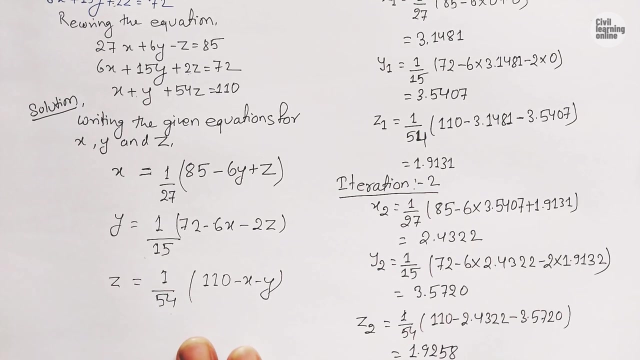 we will do. z2 equals to 1 upon 54 times 110 minus x is 2.4322. minus y is 3.5720. so here we will have 1.9258. it was for z2. similarly, we will do the third iteration and you can see the difference. 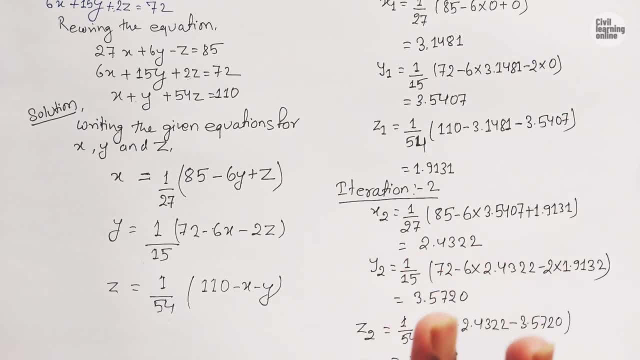 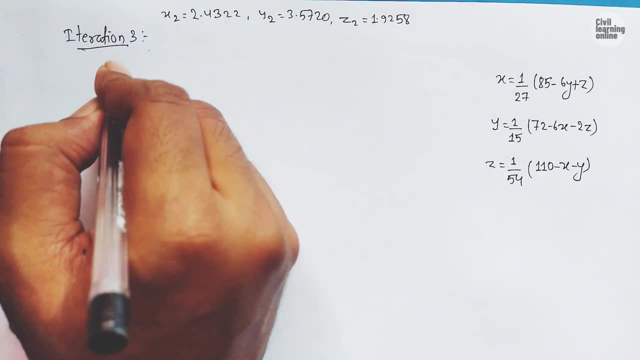 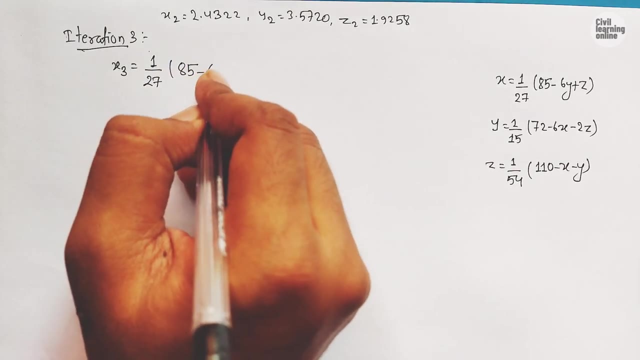 here we have 3.14, here it is 2.43. let's check if we get the similar value for iteration 3 in iteration 3 or not. now time for iteration 3, so i am going to write here: x3 equals to 1 upon 27 times 85 minus. 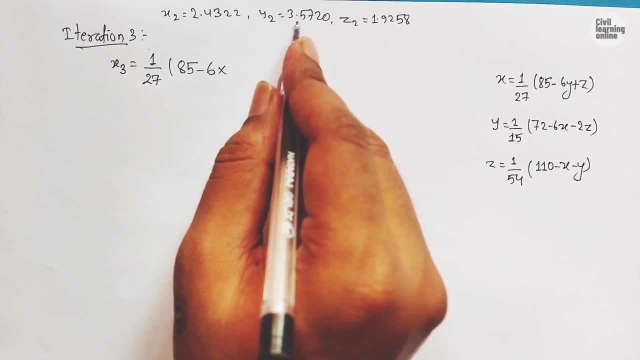 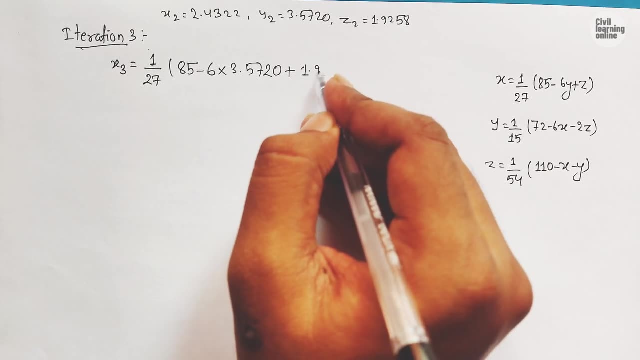 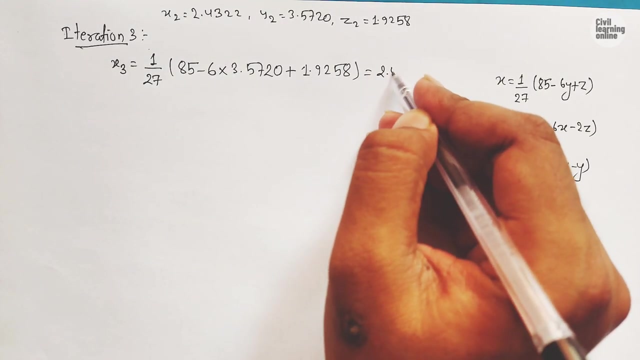 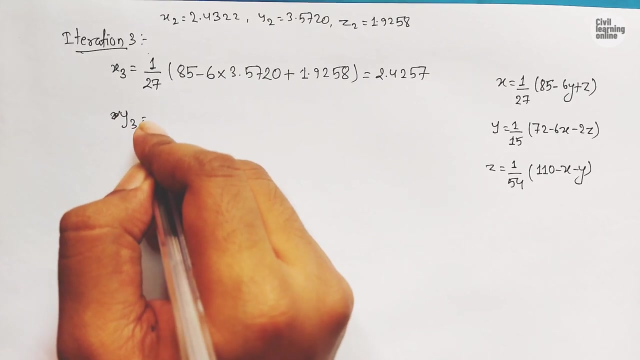 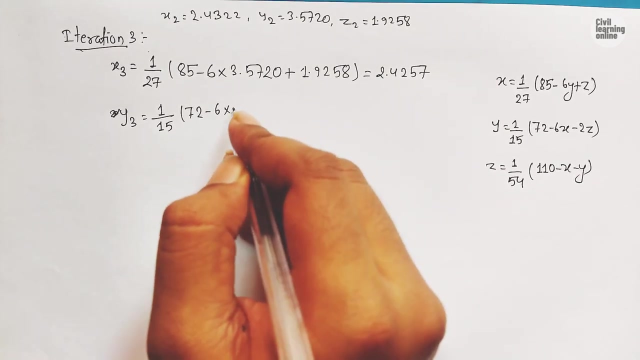 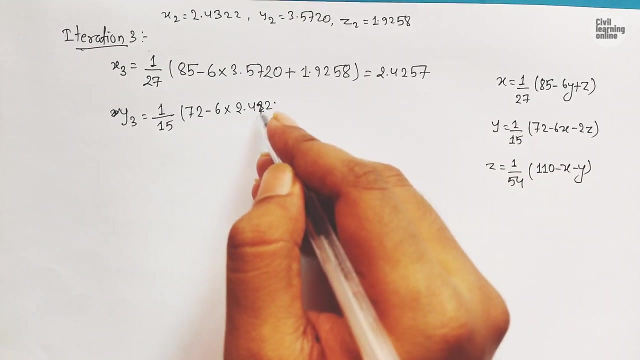 6 times y and the recent value of y was 3.5720. plus z is 1.9258 and that is equal to 3.og usf in our mommyogy for z post x. then we are going to calculate y, air and air votes with value of Matt e-mail. 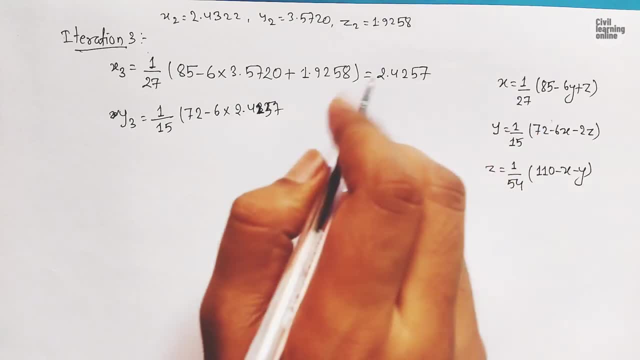 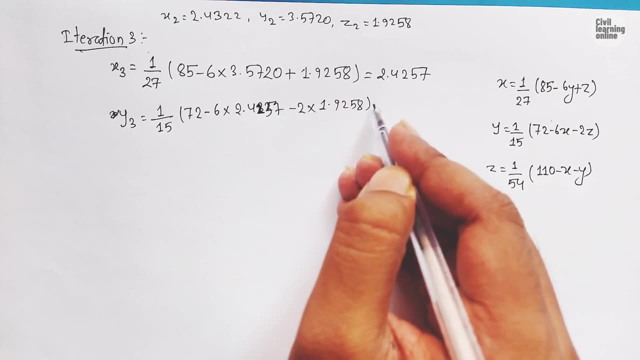 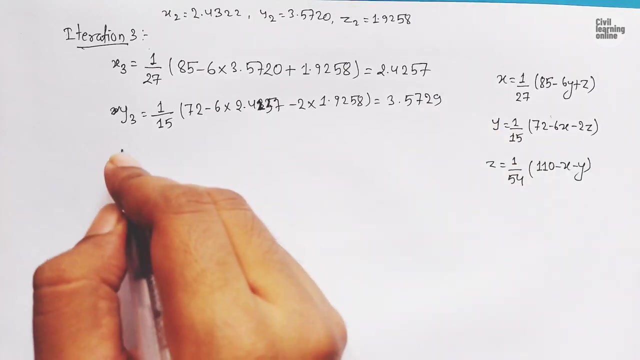 okay, we will use this value instead in place of x, and minus 2 times z, z is 1.9258. on solving this, we will get the value of y3 as 3.5729. again for y4. sorry, z3. again for z3, we will have. 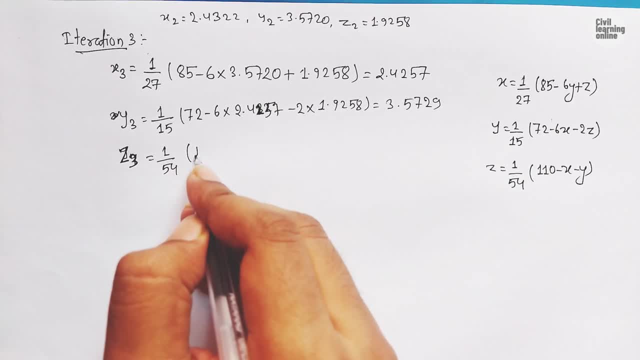 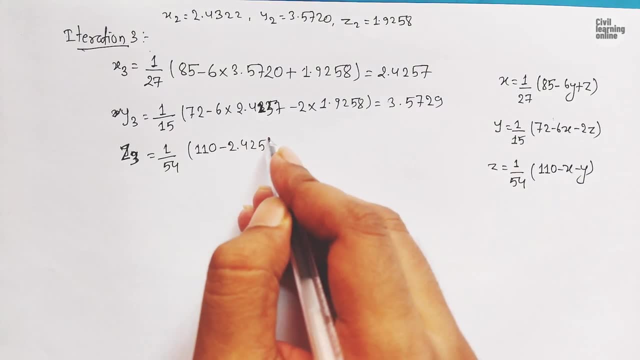 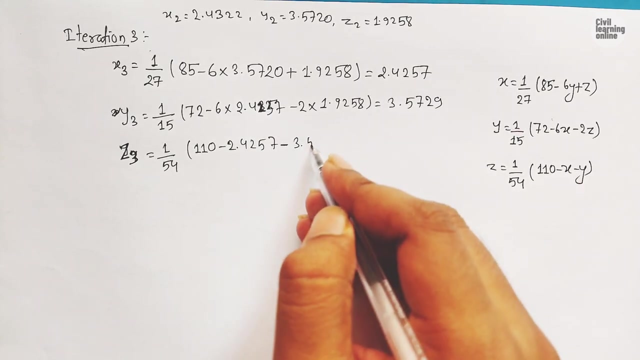 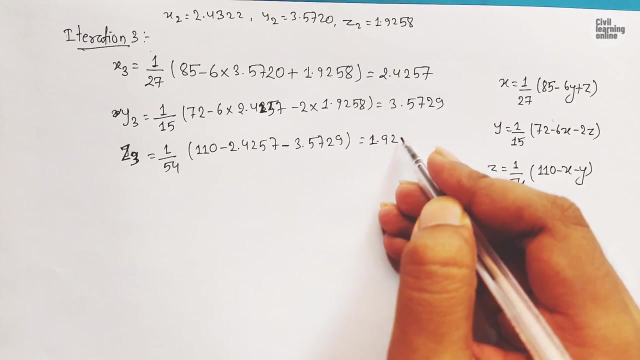 1 upon 54 times 110 minus x and x value is 2.4257 and minus y, y is 3.5729. on solving this, we will get the value of z3 as 1.9259. okay, similarly, we will do the iteration. 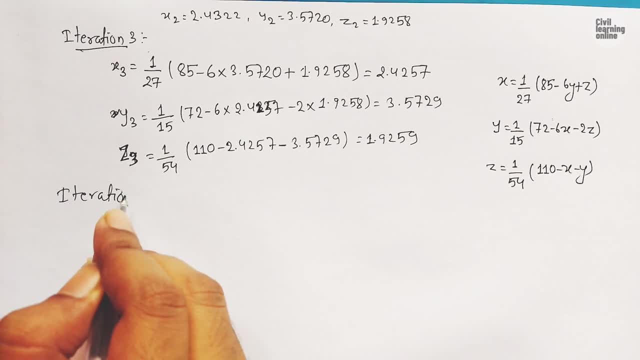 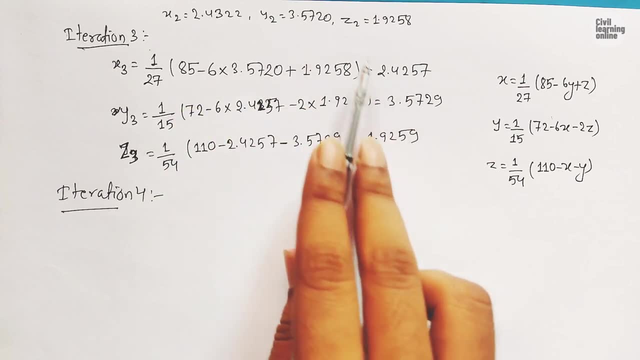 4. iteration 4 and check whether the values are getting equal or not, similar values or not. so here the value of x3 is varying from iteration 2, so we will do one more iteration and check if we are getting the similar, same value or not. in two respective iteration we have got 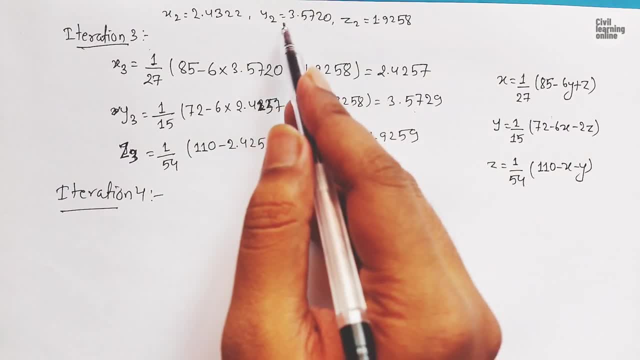 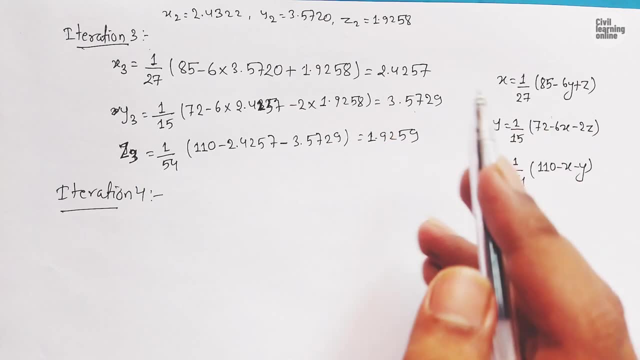 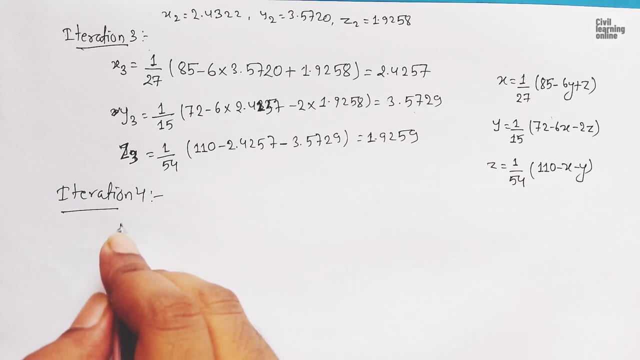 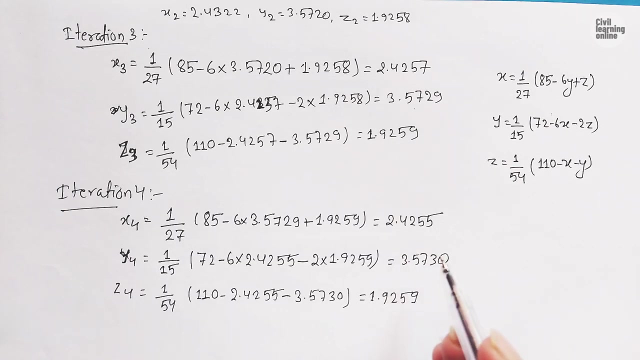 a little bit similar value of y3 and y2 in the iteration, third and second ah, and the value of z3 and z2 is a bit different ah due to four, four decimal places. so we will do the fourth iteration quickly and for fourth iteration we have. so here ah in iteration. 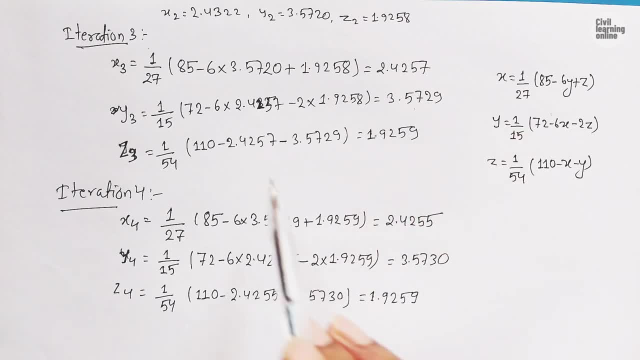 four we have get. we have got value very much close to what we have got in iteration three, see here. two point five, seven, three, zero. it is two, nine. on round off we will get three, zero, one point nine, two, five, nine. one point nine, two, five, nine. two point four, two, five. 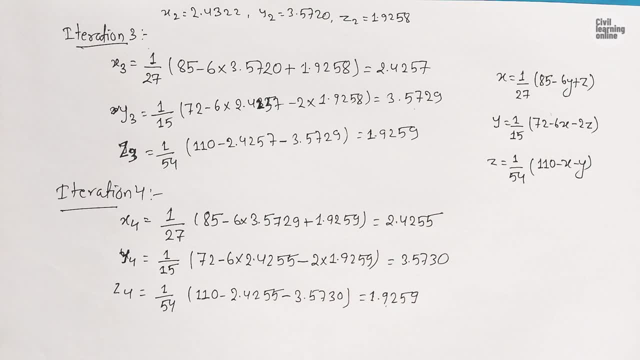 seven, two point four, two, five, five. it is similar, it can be considered equal value means the answer could be: ah, we can stop here. if not, if you still have doubt, then you can do one more step, ah, one more iteration to get to, to be more. very much confirm if you, if only. 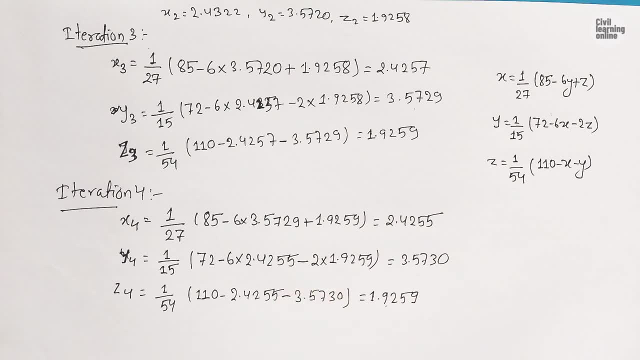 if you have exact time, extra sufficient time in exam, ok exam. if not, you can stop up to iteration four. and the benefit of using the gauss-seidel iteration method and comparison to gauss-zachowicz iteration method is that in gauss-zachowicz iteration 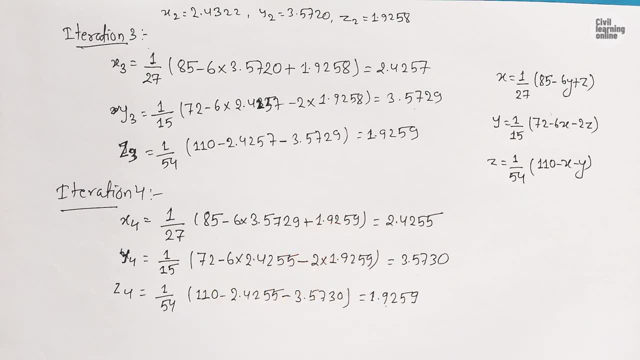 method as we are taking uh initial value. we are taking the uh in starting. we are beginning with taking x, not equals to zero, y not equals to zero, zero not equals to zero. uh it we have to do very much mean lots of iterations, you know. but in uh gauss-seidel iteration method, as we are taking, 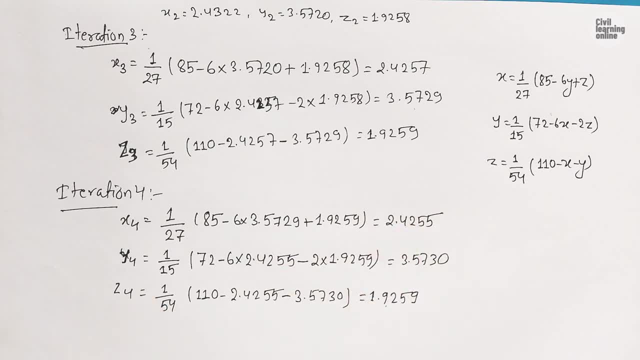 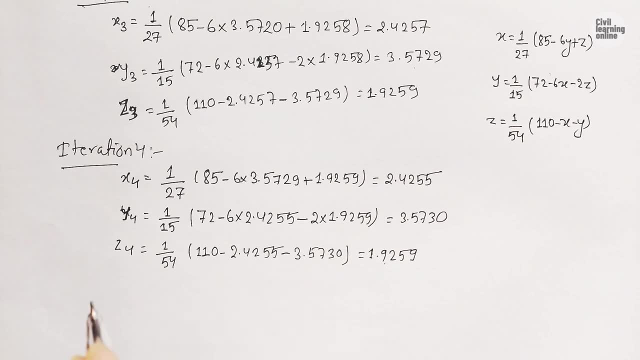 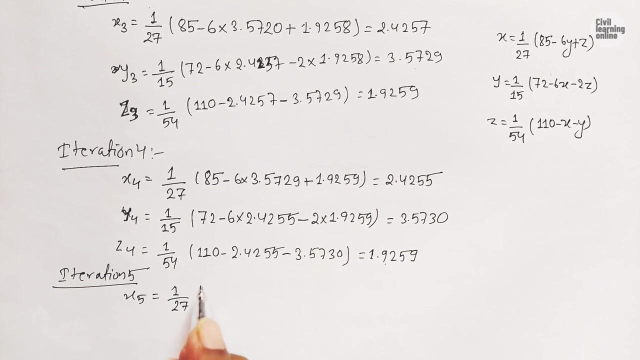 the recent value, uh, the number of hydration decreases. so here we have got the answer in fourth iteration only. if you ask me to do the fifth iteration, then see, see how we can do the fifth iteration, iteration five. so our iteration five for x five will be one by twenty seven times. 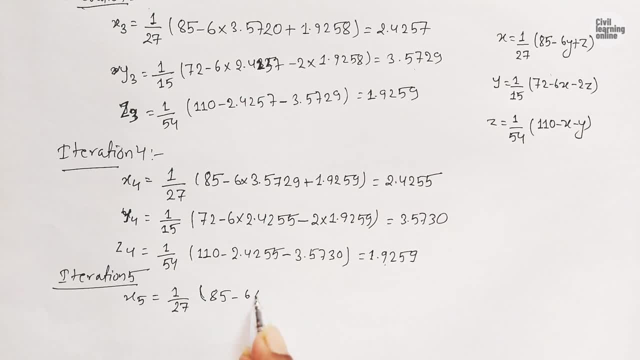 one by twenty seven times eighty five minus six times three point five. seven. three zero plus one point nine. two five nine. we will not get any kind of differences here. so two point four, two five five. similarly, we have y five equals two. this is just to, uh, show you that we are not getting any kind of differences further. so this is going to be our. 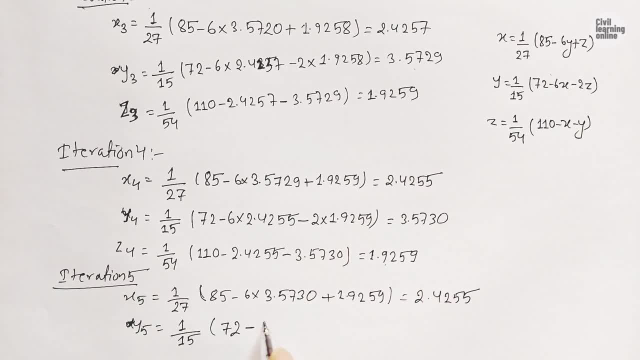 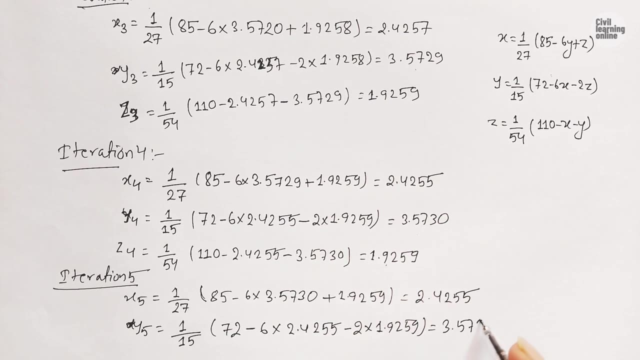 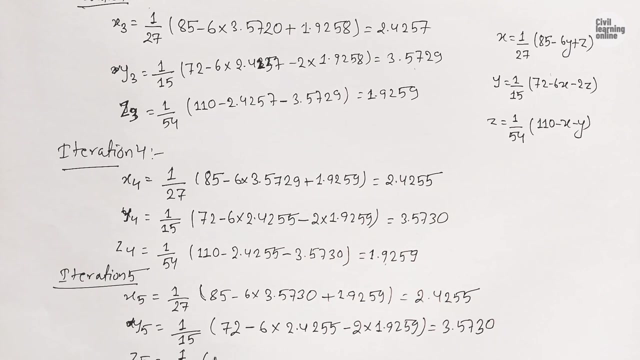 answer for x, y and z: seventy two minus six times two point four, two five, five minus two times one point nine, two five, nine. so here we will get three point five, seven, three, zero. similarly, z five will be one by fifty four times one: one zero minus two point four, two, five, five minus three point five, seven, three zero. on solving this we: 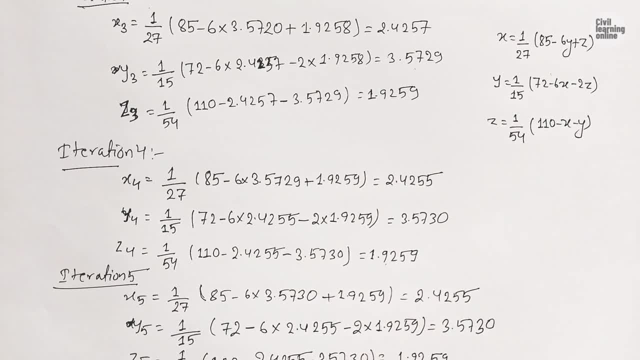 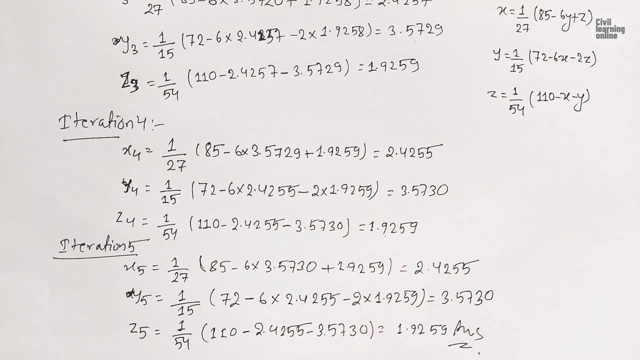 one point nine, two five nine. this is our answer. i hope you enjoyed this today's lecture. i hope- and i hope this is visible to you now- and if you are, you guys are enjoying the content and civil learning online channel, then do like this video, leave a comment if you are enjoying the content to share.